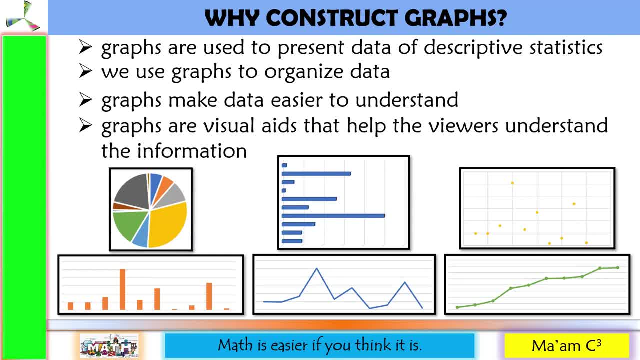 Why do we have to construct graphs? Graphs are used to present data of descriptive statistics. We use graphs to organize data. Graphs make data easier to understand And graphs are visual aids that help the viewers understand the information. Let's have the first one, the bar graph. 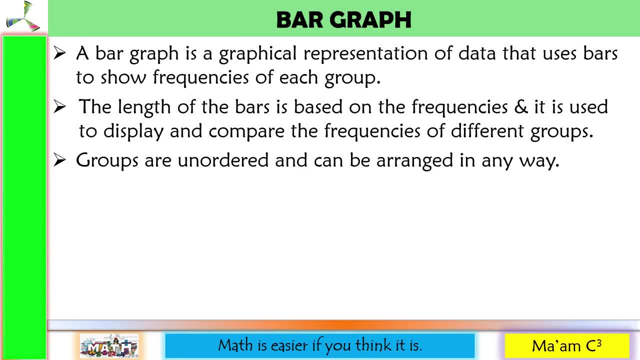 A bar graph is a graphical representation of data that uses bars to show frequencies of each group. The length of the bars is based on the frequencies and it is used to display and compare the frequencies of different groups. Groups are unordered and can be arranged in any way. 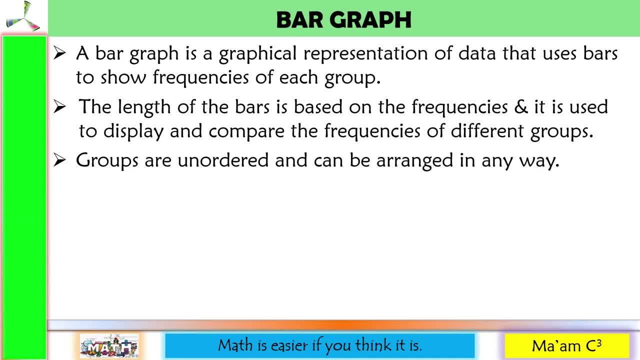 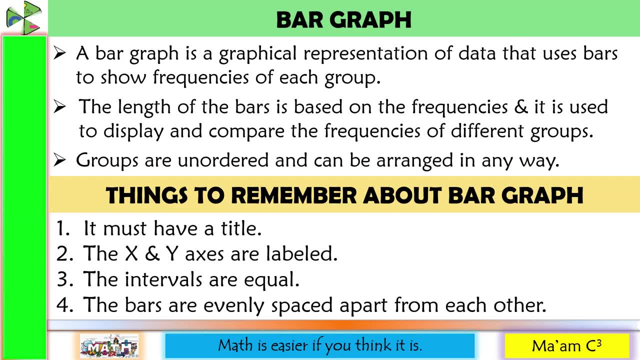 It could be alphabetical, by size or whatever you wish to be arranged. Here are some things to remember about bar graphs. Number one: it must have a title. Two: the x and y axis are labeled. Three: the intervals are equal. 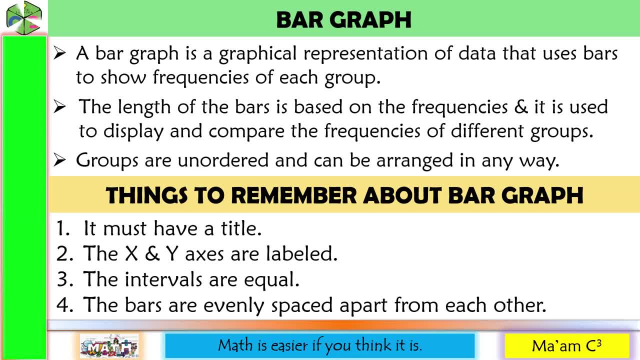 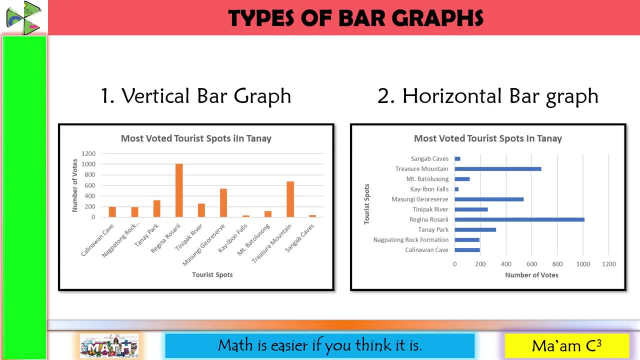 And four. the bars are evenly spaced apart from each other. There are two types of bar graphs: the vertical and horizontal bar graphs. The vertical graph displays better than the horizontal. The horizontal bar graph is useful when names are too long to fit at the foot of the column, just like this one. 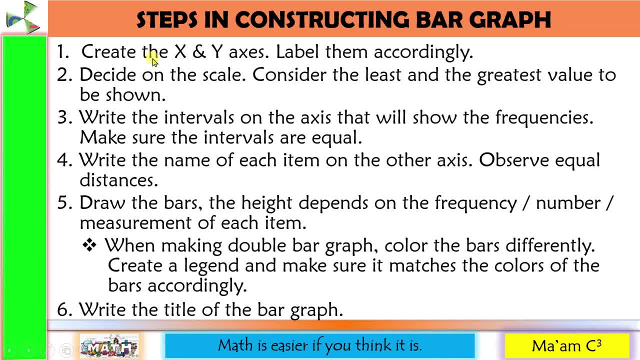 Here are the steps in constructing bar graphs. I will discuss this in detail with an example, But let me pay attention to this: When making double bar graphs, color the bars differently, Create a legend and make sure it matches the color of the bars accordingly. 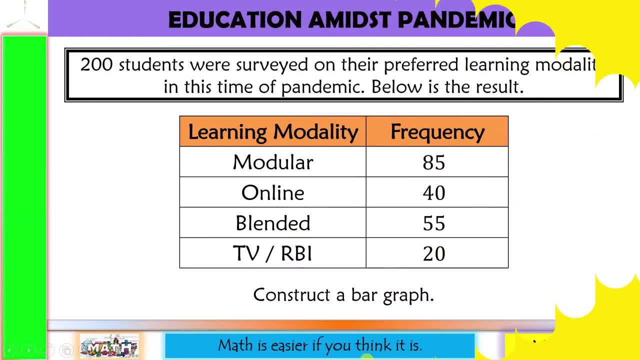 I'll show an example of this later. Let's have the example Education amidst pandemic. 200 students were surveyed on their preferred learning modality in this time of pandemic. Below is the result. Here are the different learning modalities and its corresponding frequencies. 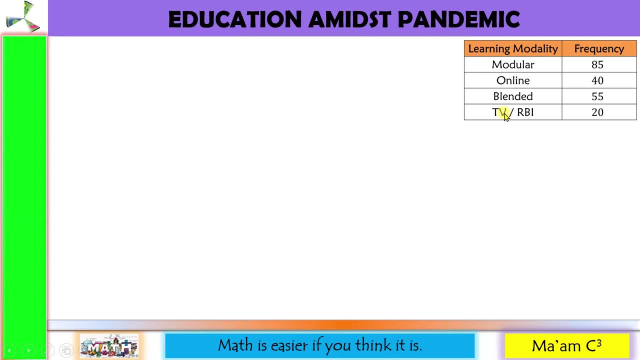 Now let us construct a bar graph. Again, here is our data. Step one: Create the X and Y axis. So we have the X axis and Y axis. Label them accordingly. I decide that the learning modality will be on the X axis and the frequency on the Y axis. 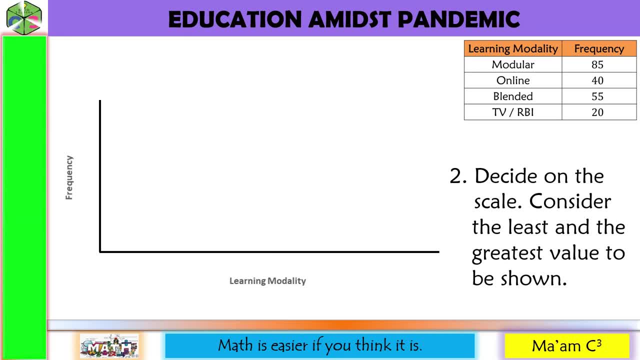 Step two: Decide on the scale. Consider the list and the greatest value to be shown. My list value is 20 and my greatest value is 85. For the scale, I'll make it by 10.. Step three: Write the intervals on the axis that will show the frequencies. 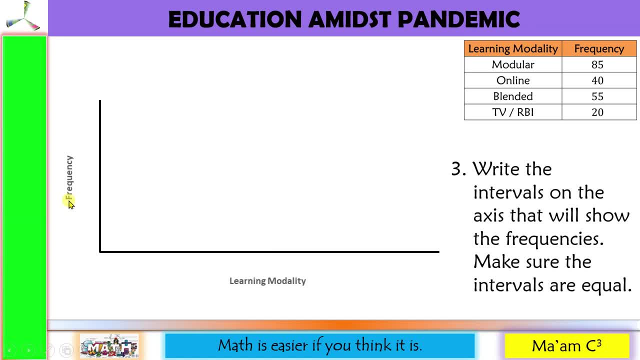 Make sure the intervals are equal. So here is the frequency. The intersection of the axis is 0.. And then my scale is 10.. So the next value is 10.. Then 20,, 30,, 40,, 50,, 60,, 70,, 80.. 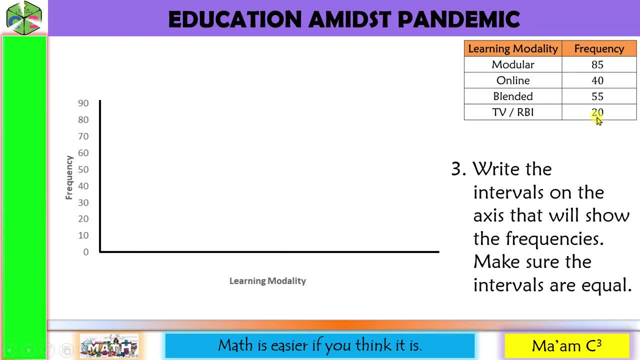 And 90. Notice that the list value, which is 20, and the greatest value, which is 85,, is covered in my frequency intervals. Next one is step four. Write the name of each item on the other axis. Observe equal distances. 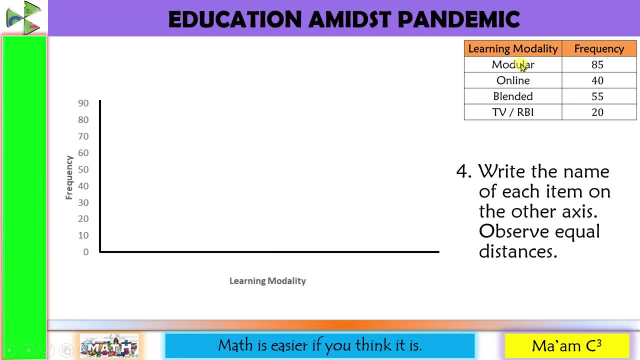 So here is the other axis. The name of learning modalities are: We have modular, online blended TV or radio-based Instruction. Step five: Draw the bars. The height depends on the frequency or number or measurement of each item. 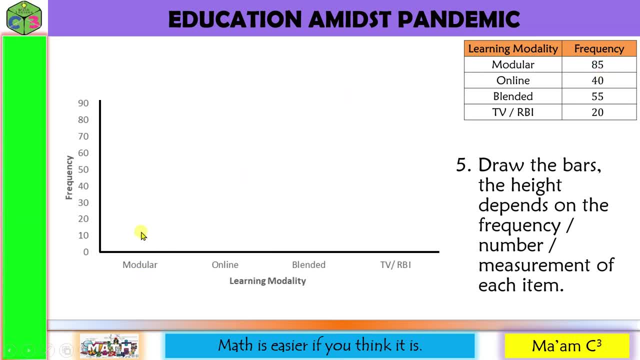 So for the modular, our frequency is 85.. So our bar graph will be up to here. For online, we have 40.. So up to here. For blended, we have 55.. For TV or radio-based instruction, we have 20.. 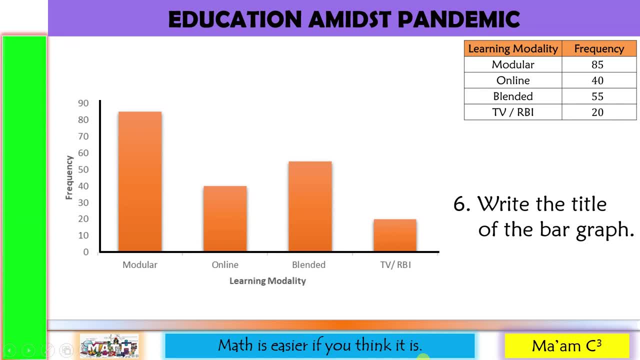 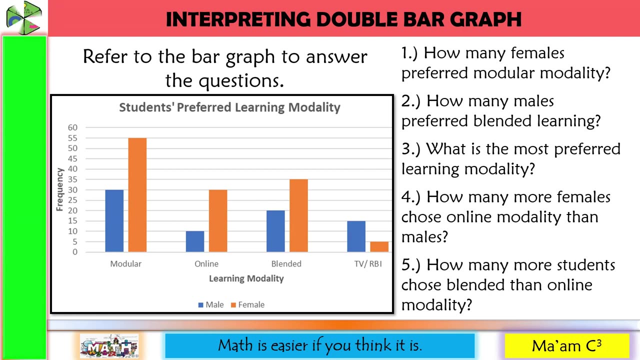 So up to here. Step six: Write the title of the bar graph. So the title of this is Students' Preferred Learning Modality. Suppose we were able to get the number of females and males in our example earlier. And here is the bar graph. 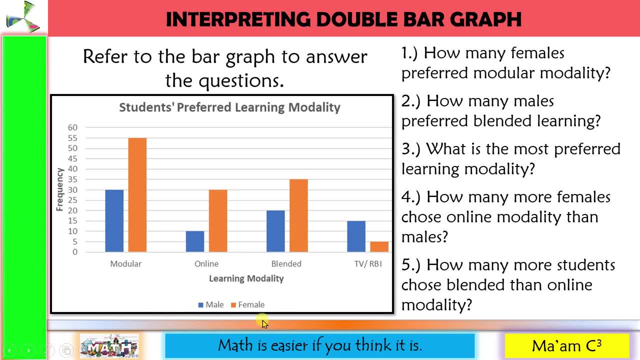 This is the legend I'm talking about earlier. When you create double bar or multi-bar graph, choose different colors and make sure the legend corresponds to the color of the bars. Now let us answer these questions. Number one: How many females preferred modular modality? 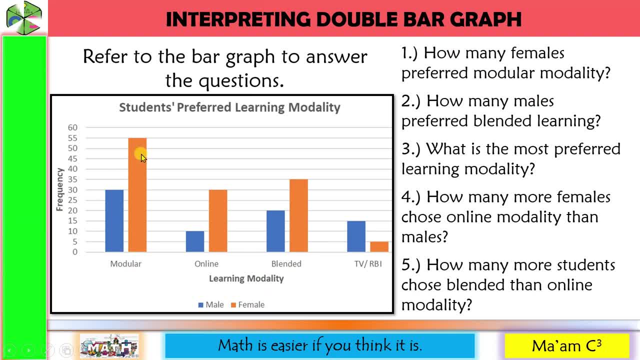 Female is color orange and then modular. Let's take a look, And there are 55 females. Number two: How many males preferred blended learning? So male is color blue and then blended. Let's see, That is 20.. Number three: 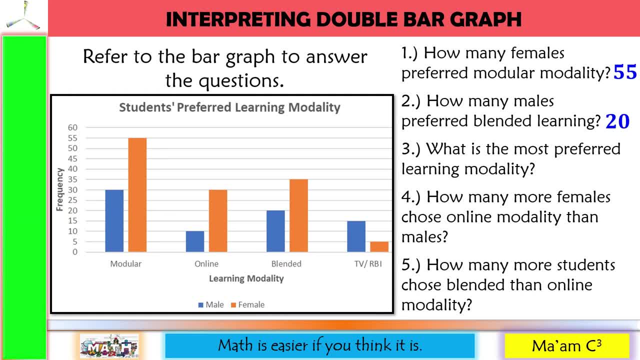 What is the Most preferred learning modality? To answer this question, we have to add the votes of male and female. So for modular, we have 30 males and 55 females. That would be 85.. For online, we have 10 males and 30 females. 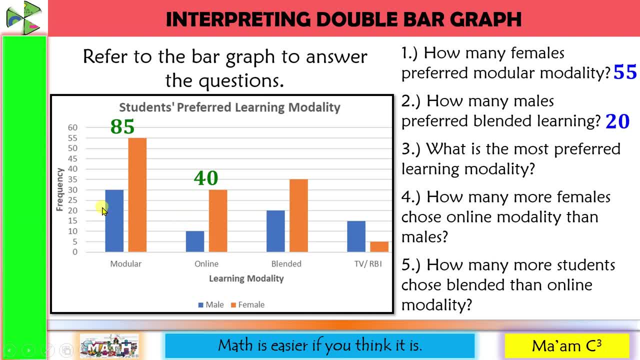 That would be 40.. For blended, we have 20 males and 35 females. That would be 55.. For TV or RBI, We have 15 males and 5 females. That would be 20.. So the most preferred learning modality is modular. 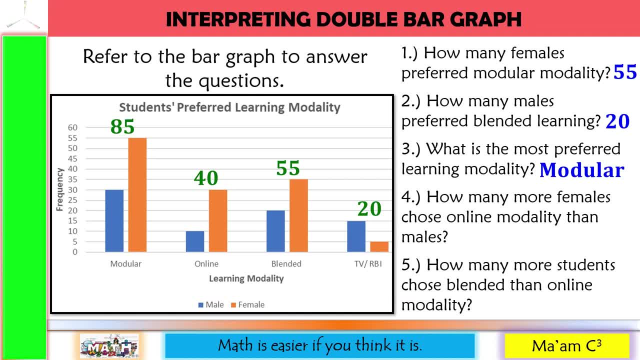 85 votes. Number four: How many more females chose online modality than males? So online females is 30, male is 10. So 30 minus 10, we have 20.. Number five: How many more students? 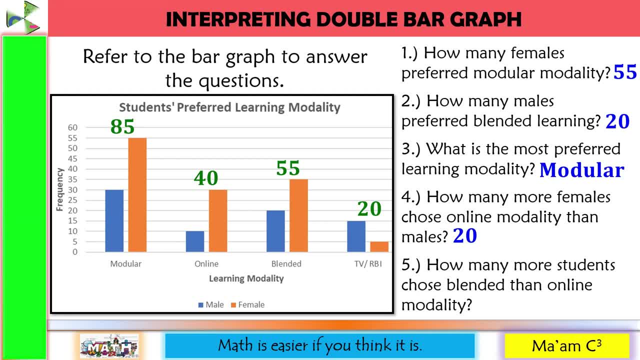 Chose blended than online modality. So we're going to compare blended and online modality. So unblended we have 55.. On online, we have 40. 55 minus 40 is 15.. So 15 more students preferred blended than online modality. 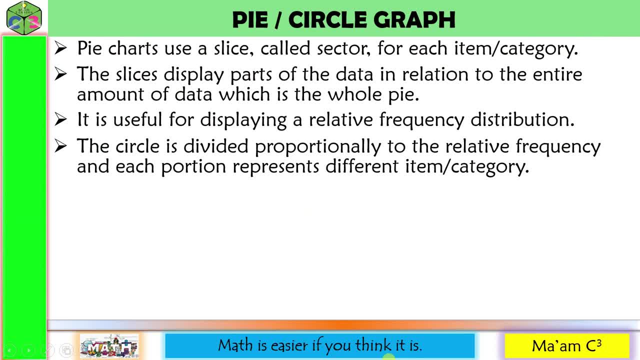 Let's have the second graph, The pie or circle graph. Pie charts use a slice- It's called sector- for each item or category. The slices display parts of the data in relation to the entire amount of data, which is the whole pie. 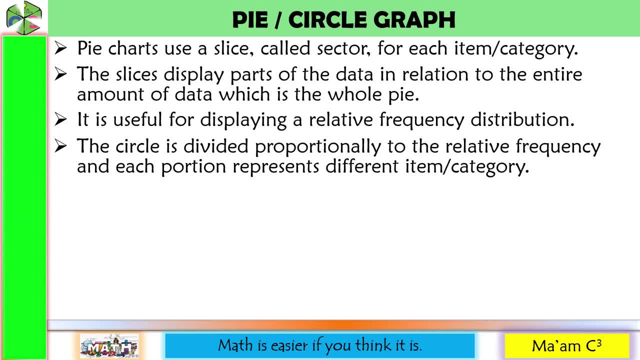 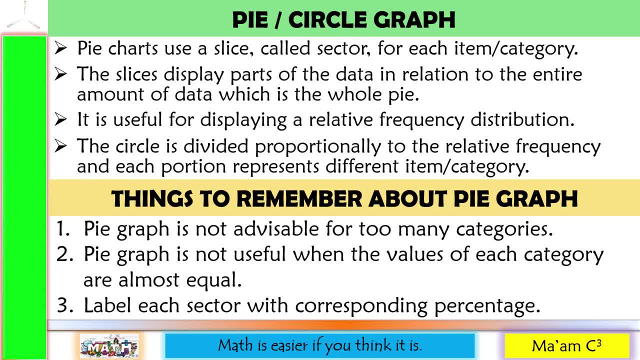 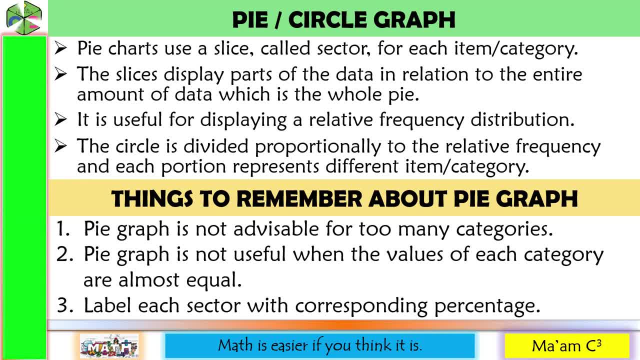 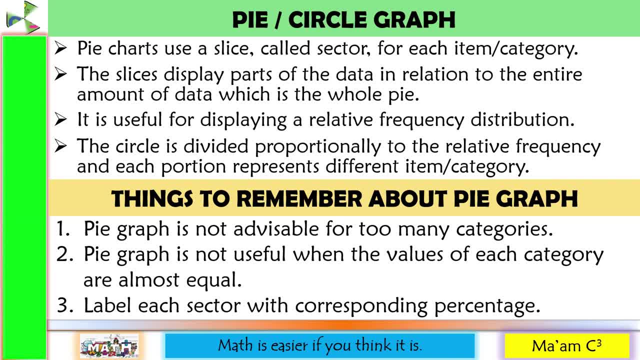 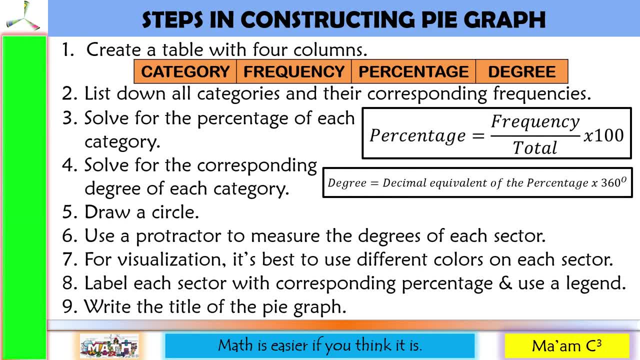 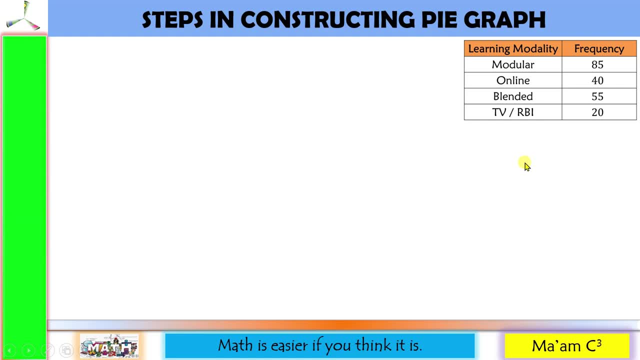 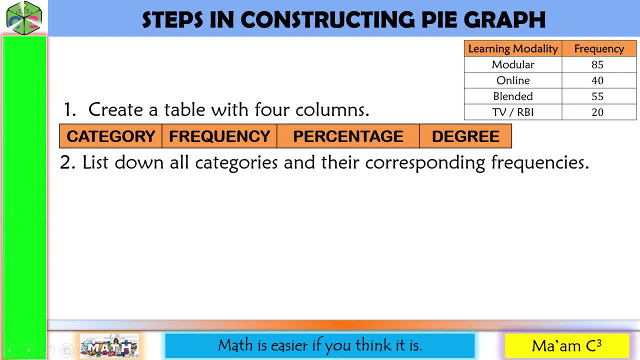 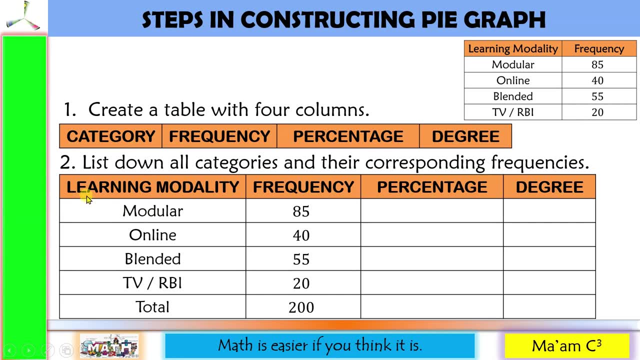 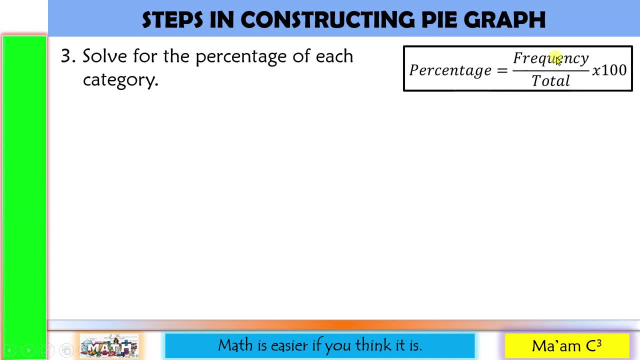 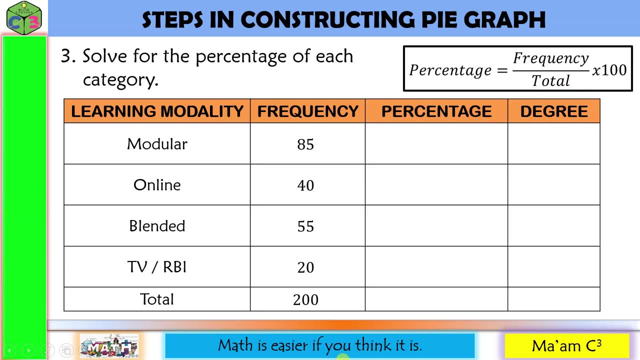 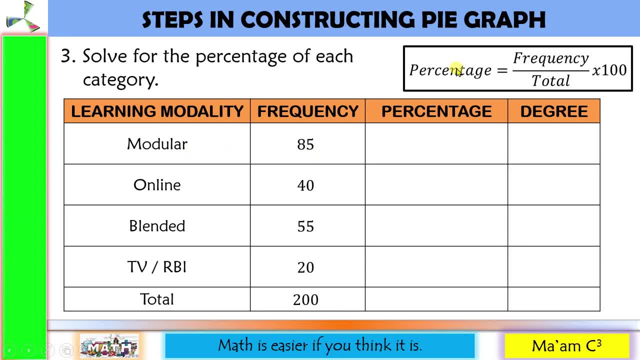 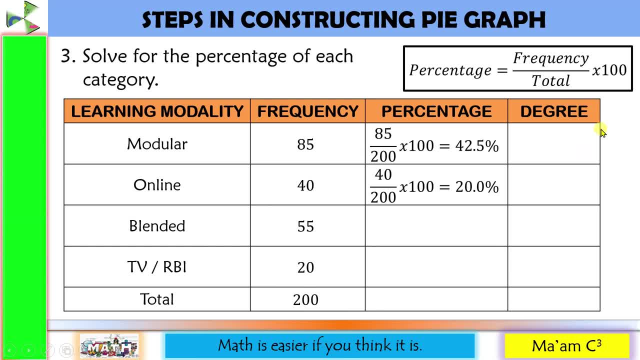 for blended, we have: 55 divided by 200 times 100 is equal to 27.5 percent. and the last one, 20 divided by 200 times 100 is equal to 10 percent. to check, sum up all the percentages. this should be equal. 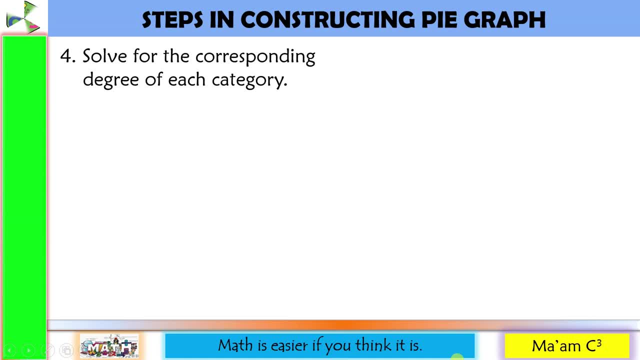 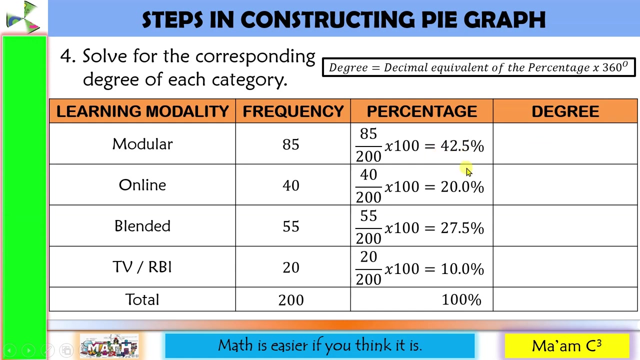 to 100, step 4: solve for the corresponding degree of each category. here is the formula: the degree is equal to the decimal equivalent of the percentage times 360 degrees. so again, our table for the degree. first we're going to get the decimal equivalent of this. to do that you just have to move the decimal point. 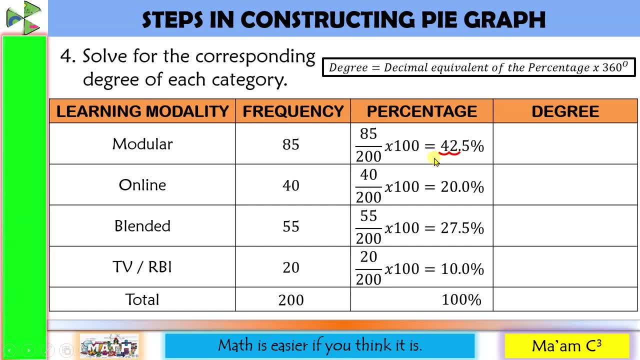 two places going to the left, so this is equal to 0.425. and then times 360 degrees and this is equal to 153 degrees. so for online, again move the decimal point two places going to the left, that would be equal to 0.2. 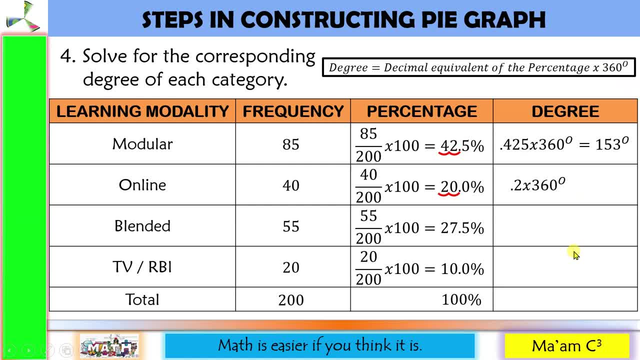 times 360 degrees, and that is equal to 72 degrees. for blended: again move the decimal point two places going to the left: this is 0.275 times 360 degrees, is equal to 99 degrees. and last one, this will be 0.10 times 360 degrees and that is equal to 36 degrees. to check, sum up all the percentages: 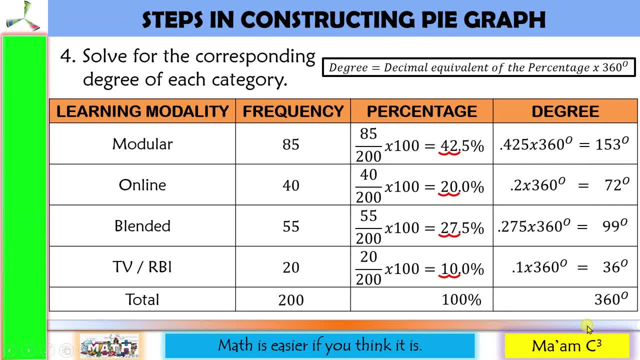 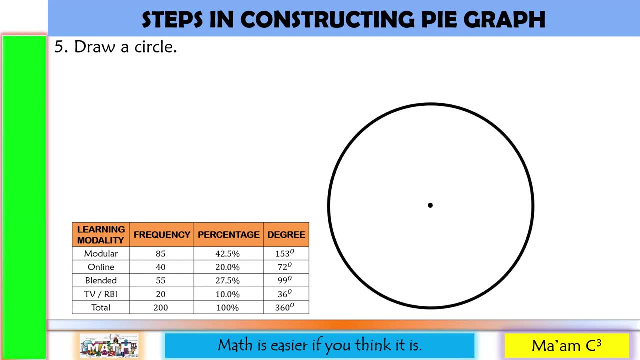 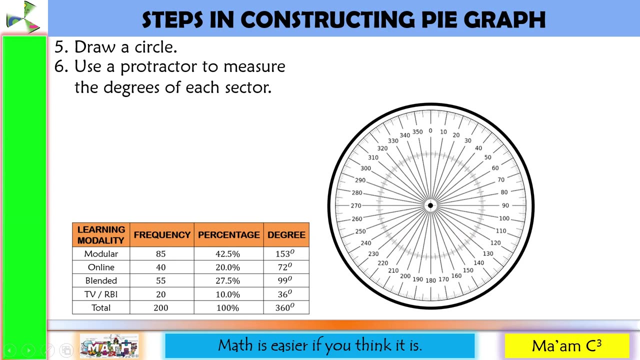 sum up all the degrees. it should be equal to 360 degrees, because one complete circle measures 360 degrees. step 5: draw a circle. let us locate the center. step 6: use a protractor to measure the degrees of each sector. so i'm going to use 360 degrees protractor here. 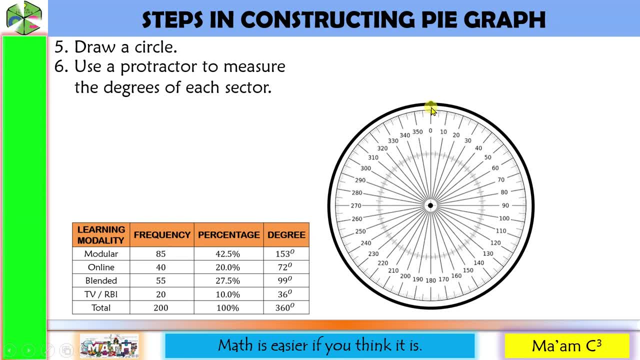 using the protractor. here the detachment is: apply the detachment and measure the dropped�� is theoweenen 무슨 perspective of each sector. so i'm going to use 360 degrees protractor here. Since my zero is here, I'm going to create a point here. 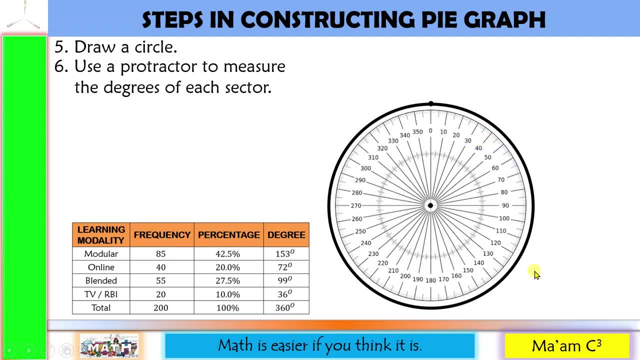 The first one is 150 degrees, So that is in here. And then 150 degrees plus 72 degrees is equal to 225.. So it will be here. And then 225 plus 99 degrees is equal to 324.. So it should be here. 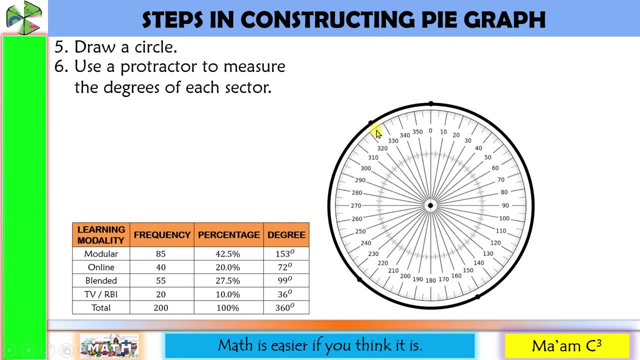 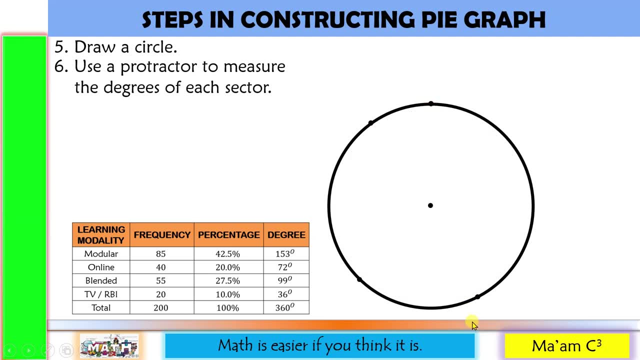 Now, 324 plus 36 is equal to 360. So that will be here. So let us remove our protractor. Let us connect our points to the center, Step 7.. For visualization, it's best to use different colors on each sector. 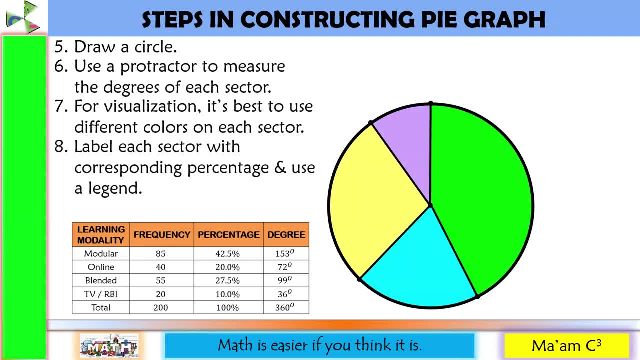 Step 8. Label each sector with corresponding percentage and use a letter. The first one that we measure has a corresponding 42.5%, And the second one is 20%. The third one is 27.5% And the last one is 10%. 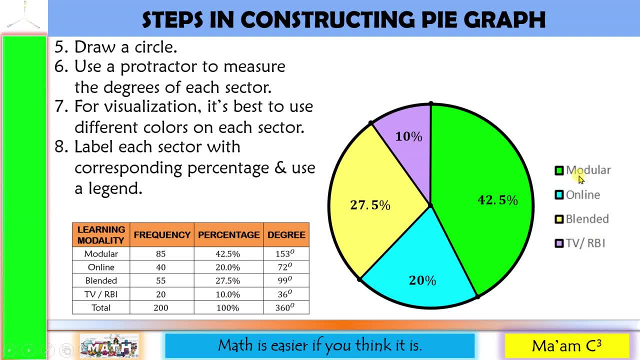 Then for the legend, we'll put it here. So: grid for modular, blue for online, yellow for blended and violet for TV or radio-based instruction. Step 9. And step 9, write the title of the pie graph. So, once again, the title of this is: 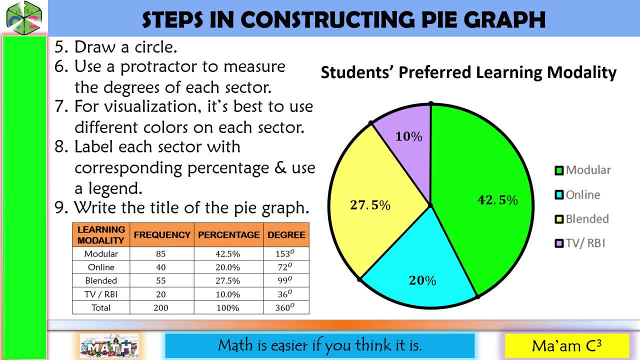 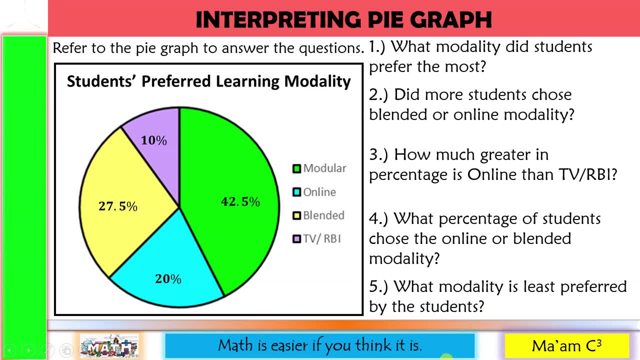 Students' Preferred Learning Modality. Now let us interpret this pie graph by answering these questions. Number 1. What modality did students prefer the most? So you can easily see that in our pie And that would be 42.5%, which is the modular modality. 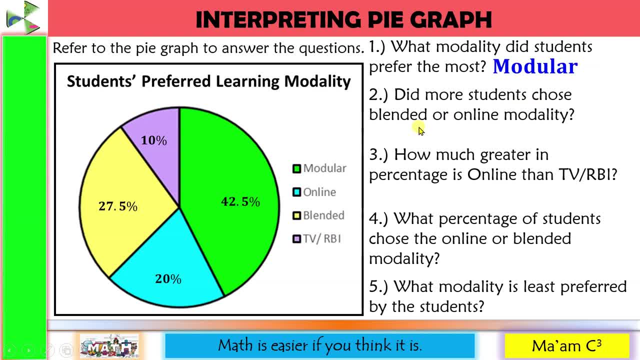 Number 2. Did more students chose blended or online learning? So we are going to compare blended yellow and online, which is blue. So which students chose more? That would be the blended learning Number 3.. How much greater in percentage is online than TV or radio-based instruction? 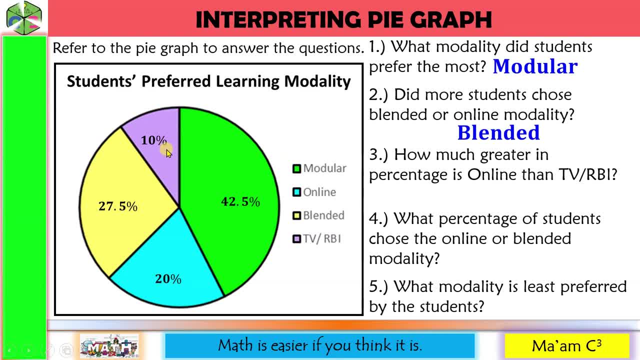 So how much greater is online than TV or radio-based instruction? 20 minus 10 is 10% Number 4.. What percentage of students chose the online or blended modality? So online is blue again and blended is yellow. So what percentage? 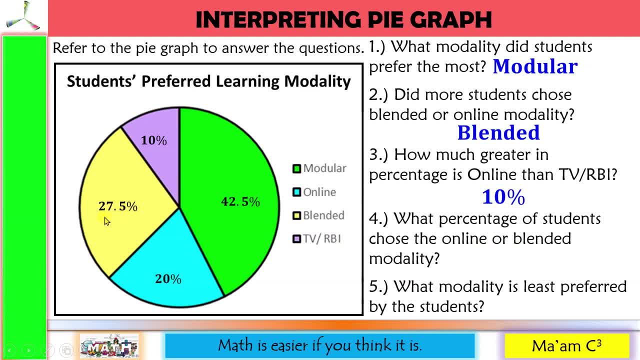 We're going to combine. It says here or So: 27.5 plus 20 is 47.5%. And last one, What modality is limited? The list preferred by the students. So you can easily see that. And the smallest percentage is 10%. 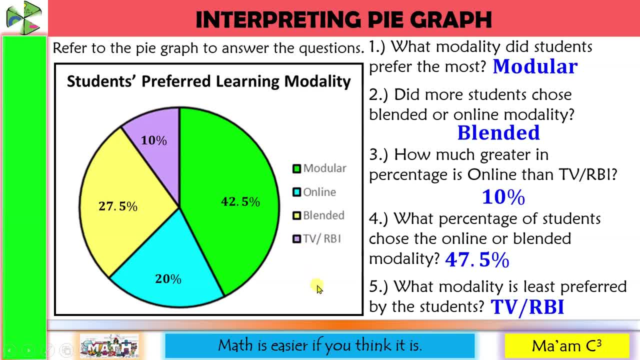 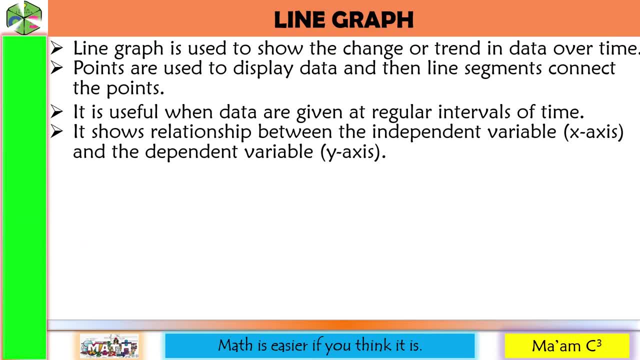 That would be the TV or radio-based instruction. Let's have the last one, The line graph. Line graph is used to show the change or trend in data over time. Points are used to display data And then line segments connect the points. 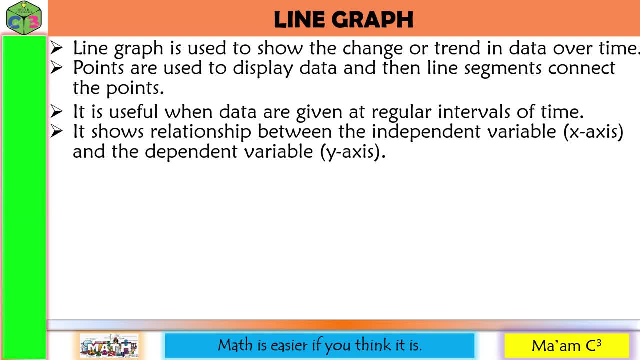 It is useful when data are given. The next one is the The last one. It shows the relationship between the independent variable, which is the X axis, and the dependent variable, which is the Y axis. Just remember, the independent variable can stand alone. 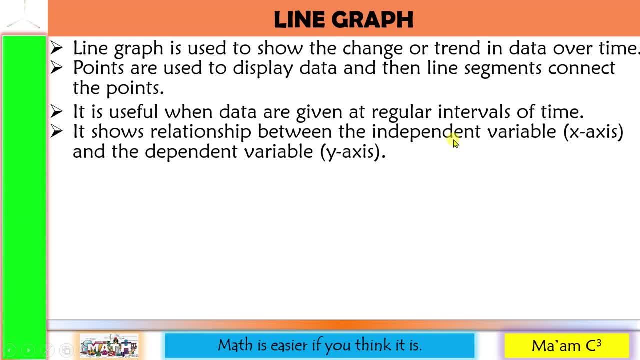 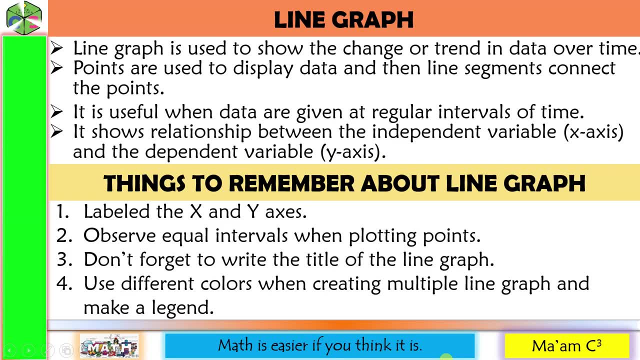 So, even without the dependent variable, the independent variable will happen. Here are some things that you need to know, That you need to remember, about the line graph Number one: label the X and Y axis. Two, observe equal intervals when plotting points. 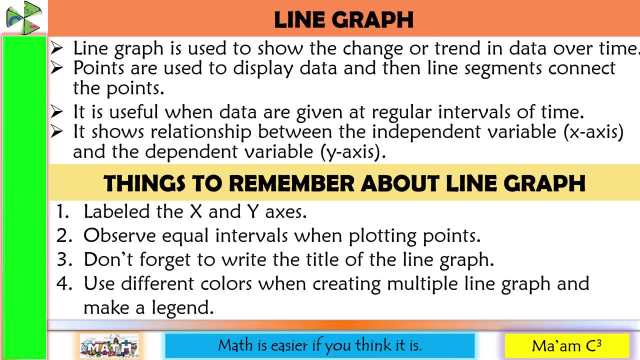 Three, don't forget to write the title of the line graph. And four, use different colors when creating multiple line graphs and make a legend. So this is the same when we create a double or multi-bar graph. Here are the steps in constructing a line graph. 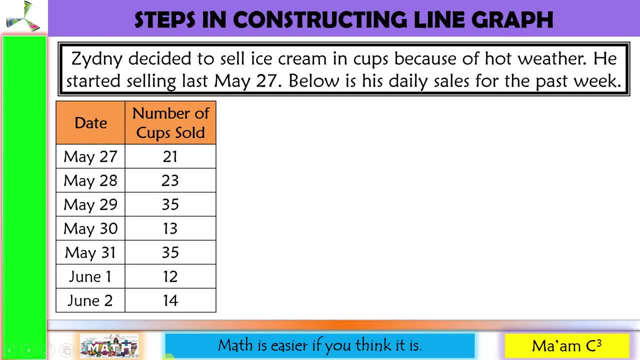 Let's have an example. Zidney decided to sell ice cream in cups because of hot weather. He started selling last May 27.. Below is his daily sales for the past week. Step one: identify the independent and dependent variable. So our independent variable, here is the date. 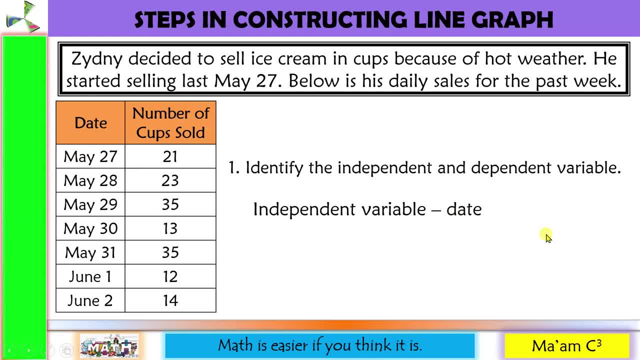 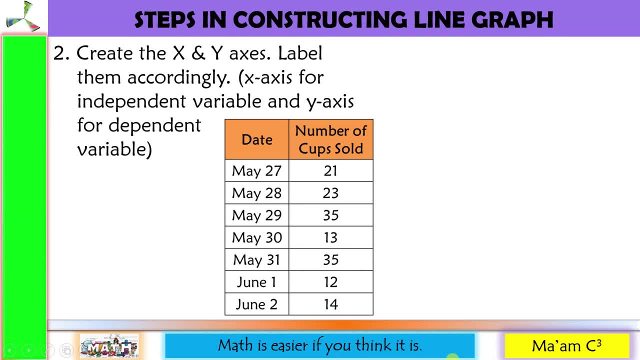 Whatever happens, the date will continue to go on And our independent variable is the number of cups sold each day. Step two: Create the X and Y axis. Label them accordingly, So we have the X axis and the Y axis. The independent variable is the date. 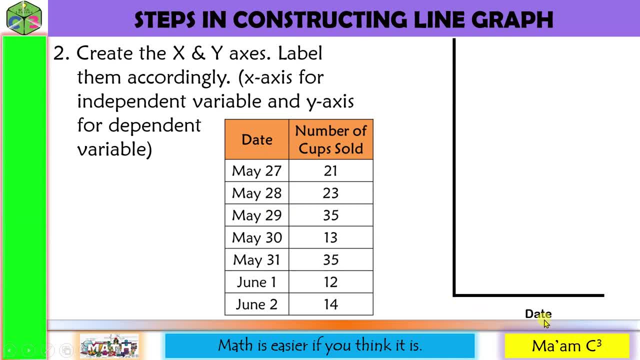 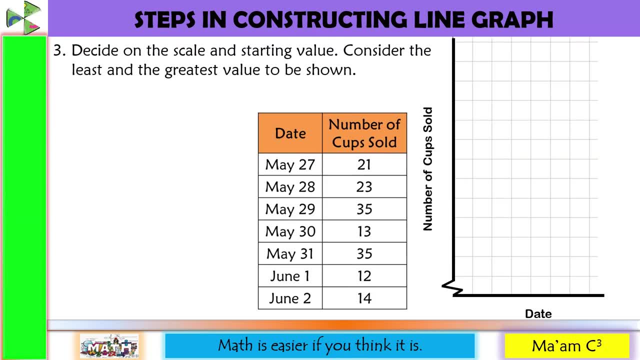 So we're going to put it here: The dependent variable is the number of cups sold, So we're going to put it here. on the Y axis. Step three: decide on the scale and starting value. Consider the list and the greatest value to be shown. 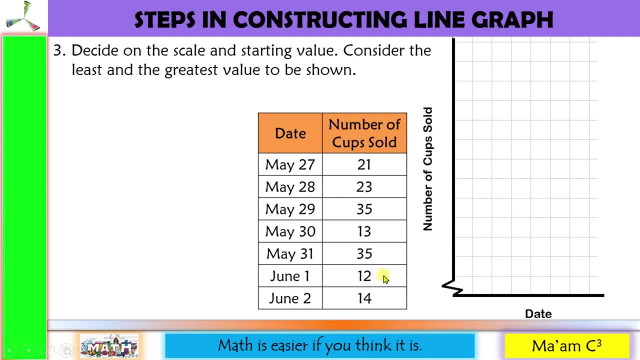 The list value is 12. And I decide that This will be my starting value. The greatest value is 35.. For the scale, I choose a scale of two as the interval. Step four: write the intervals on Y axis. Make sure the intervals are equal. 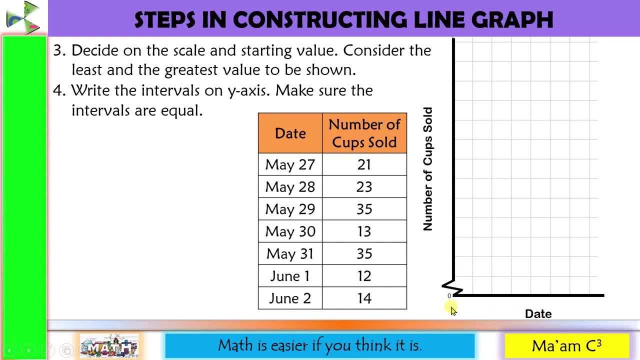 The intersection of the axis is zero. Like what I've said earlier, the list value, which is 12, is my starting value, So I'll start here with 12.. Notice this zigzag here. It represents the gap between zero to 12.. 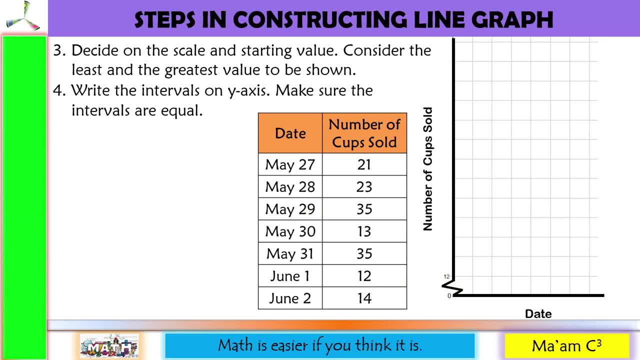 Now for the scale. I've said that I choose two as my interval. So after 12, I have 14, and then 16,, 18,, 20,, 22,, 24,, 26,, 28,, 30,, 32,, 34, and 36.. 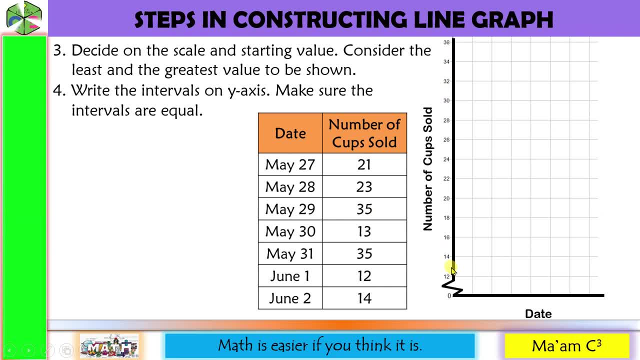 The greatest value, which is 35, is covered in my interval as well as my list value. Step five: write the name of each independent variable on the X axis. Observe equal distances. The name of the independent variable are the dates. 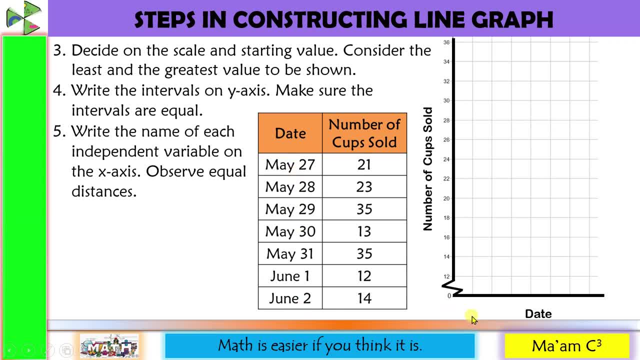 So May 27 to June 2.. I'll use number instead, So I have 527,, 528,, 529,, 530,, 531,, 61, and 62.. Step six: plot the data points. Connect them. 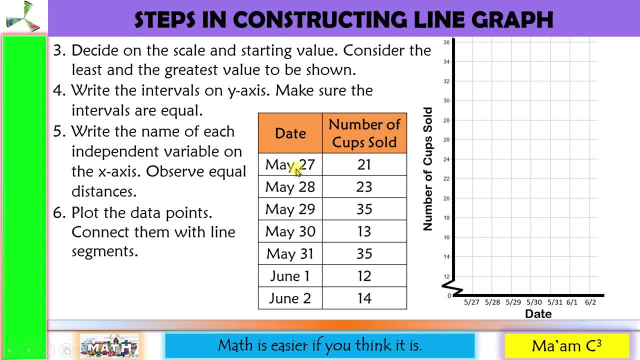 So for May 27, the number of cups sold is 21.. So May 27,- 21 is at the middle of 20 and 22. May 28,: 23 cups. So May 28,, 23,. it's here. 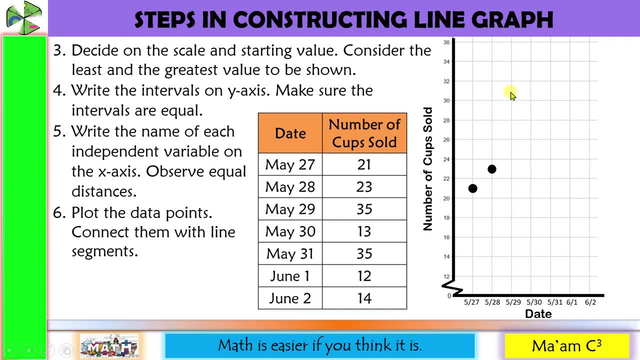 May 29, 35 cups. So 35 cups. it's here. May 30, 13 cups. May 30, 13 cups is here. May 31.. May 31. May 31,- another 35.. 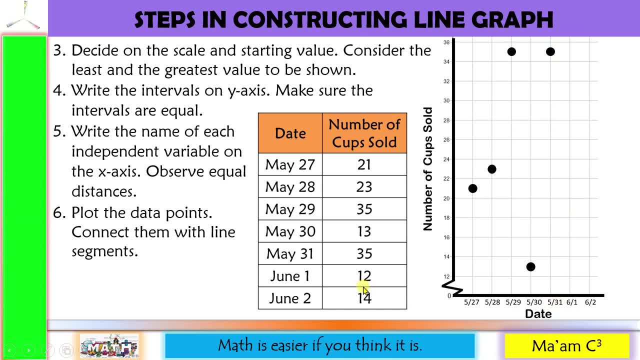 So it would be here June 1, we have 12 cups here And June 2, 14 cups here. Next, connect them with line segments. So we have 1,, 2,, 3,, 4,, 5, 6 line segments. 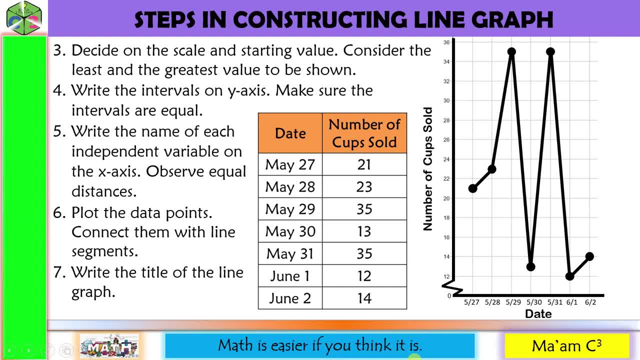 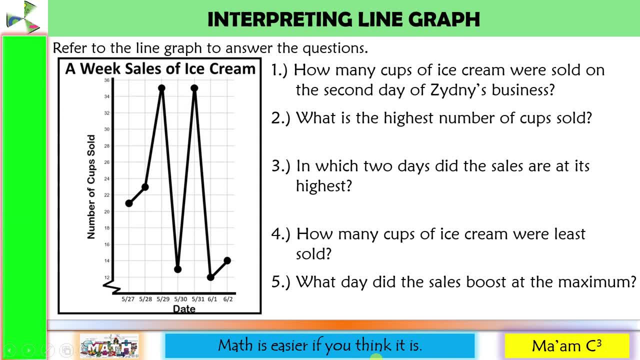 Next is step seven. write the title of the line graph. I'll just put here on top: A week's sales of ice cream. Now let us interpret this line graph: How many cups of ice cream were sold on the second day of Sidney's business? 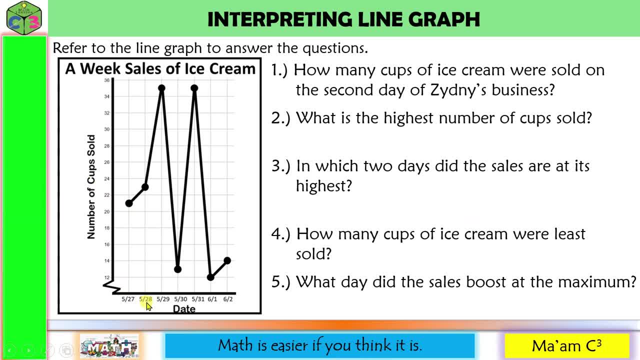 Second day, May 27, is the start. So the second day is May 28.. And he sold 23 cups. Number two: what is the highest number of cups sold? That would be 35.. Number three, in which two days did the sales, are its highest. 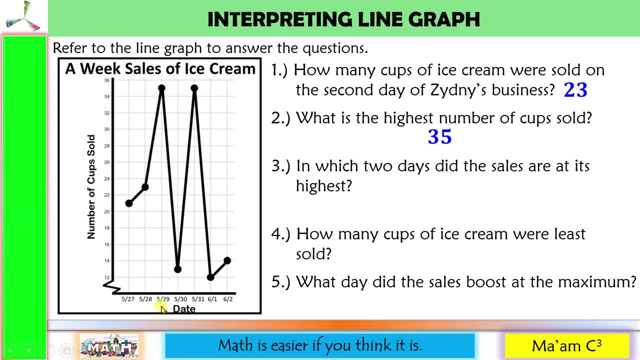 In which two days? Those are May 29 and May 31.. Number four: how many cups of ice cream were least sold? So least sold is 12 cups. And number five: what day did the sales boost at the maximum? To answer this question, we have to consider the days where there are rising trends. 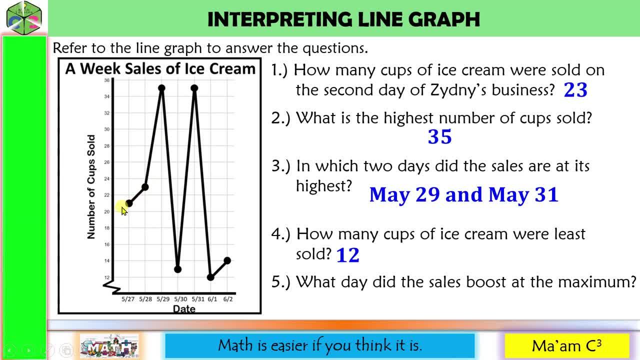 So those line segments that are going up. So for this one, 23. Minus 21 is equal to 2.. This is also rising. 35 minus 23 is equal to 12.. We're not going to consider this one. 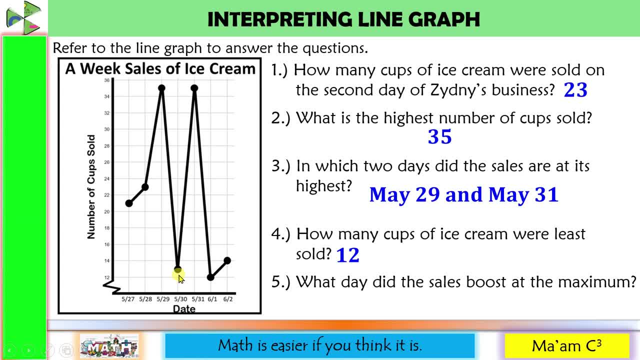 We're going to consider this: 35 minus 13 is equal to 22.. We are not going to consider this. This one is: 14 minus 12 is equal to 2.. So the biggest number in rise is on May 31.. 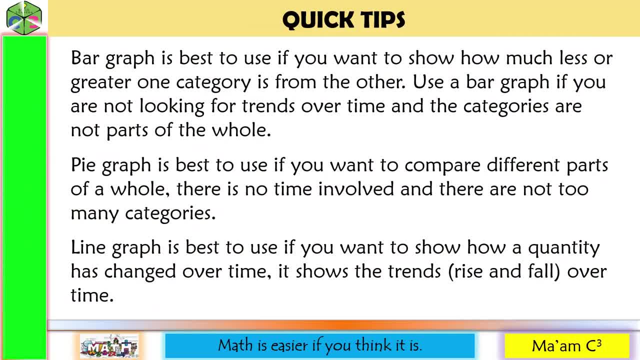 A rise of 22 cups. Quick tips. Bar graph is best to use if you want to show how much less or greater one category is from the other. Use a bar graph if you are not looking for trends over time and the categories are not parts of the whole. 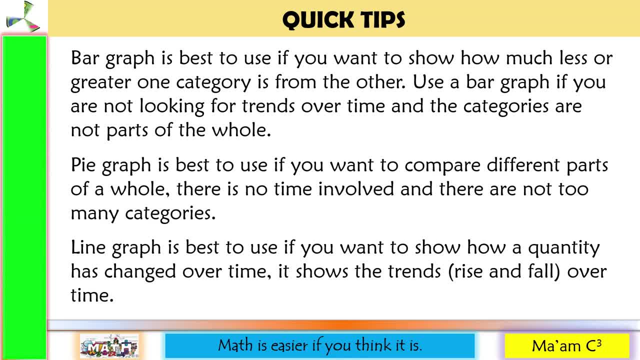 Pie graph is best to use if you want to compare different parts of a whole. There is no time involved and there are not too many categories. Line graph is best to use if you want to show how a quantity has changed over time. It shows the trends rise and fall over time.